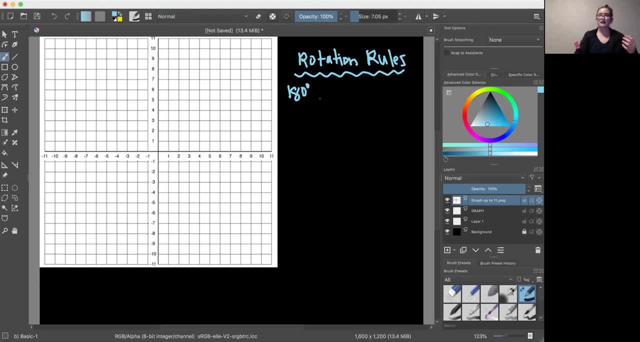 clockwise or counterclockwise, because, let's say, if this is our image, if we're going 180 degree rotation, it's going to end up over here, somewhere in this quadrant. and so if we're going this way, clockwise, we'll get there, and if we're going counterclockwise, we'll get there. 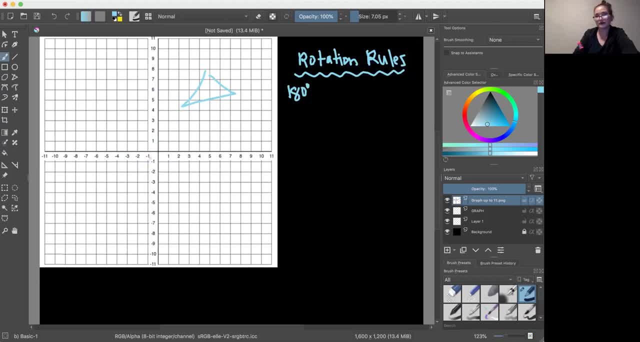 Because it's a straight line and 180 degree rotation. Okay, so it doesn't matter what direction, so I'm going to skip the direction, I'm just going to write the rule. Okay, so the rule is any point that you have: x and y is our ordered pair. It is going to still stay x and y. 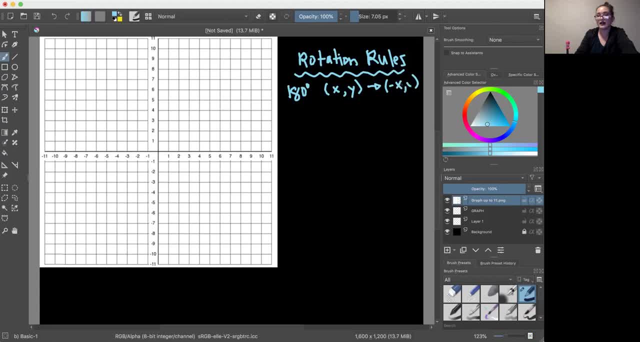 but you're going to take the opposite of x and the opposite of y. So an example- let me just make my pen a little bit small in here- but an example of that, if let's do our examples in a different color. but if I had, let's say, if I had two comma negative four as my point. 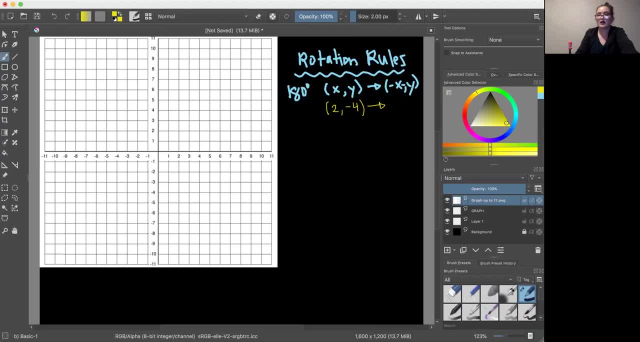 and I'm doing 180 degree rotation. I am going to still keep x and y the same, the same order: x goes first, y goes second, but it's going to be in the opposite of x. So the opposite of my two here is. 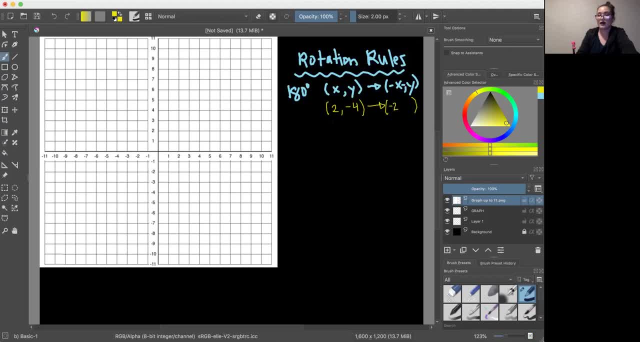 going to be negative two and the opposite of my negative four is going to be a positive four. Okay, so let's just graph that right now, just to show you what that looks like. My original point was two. where's my thing here? so my original point was two and 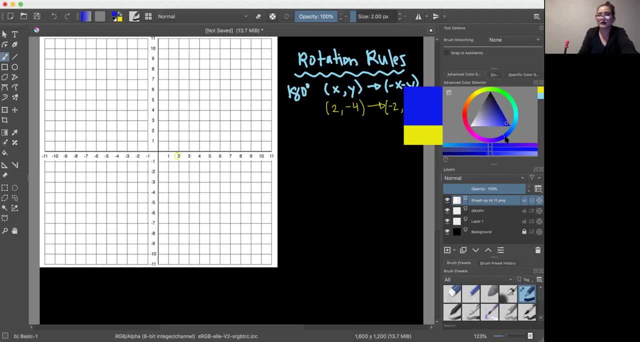 my x was two, and it's kind of hard to see in this color, so let's go back to our blue. But my original point was x was two and y was negative four, and so the point would be right here. Okay, with 180 degree rotation. my x then was negative two. if I can find my little teeny tiny. 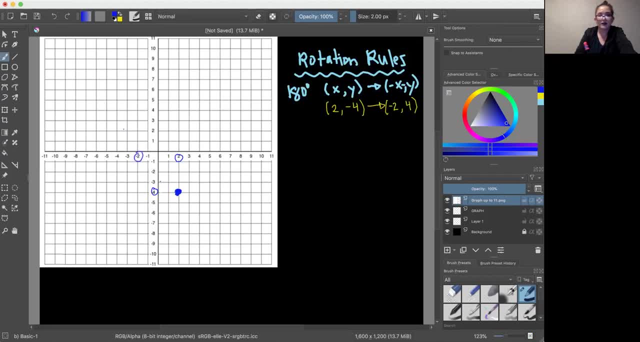 dot here. it's negative stitches here, so I can see how undersized it's going to get from that point. Okay, so right now it's because constant picking always kind of on the逆線, so if I Okay. so my x was negative two and my y then became four. so with that, 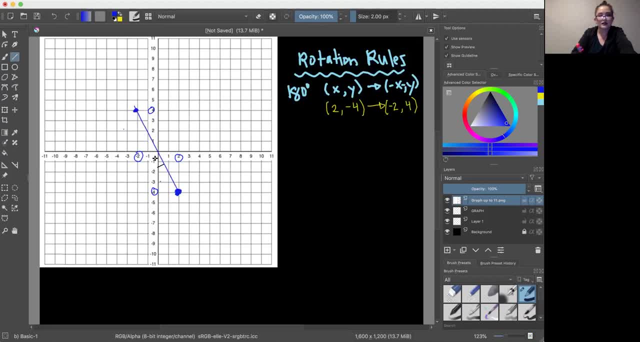 Yes, sorry I had to double check because that didn't look right. but yes, negative two comma four. I'm sorry I forgot to say about the origin, but from this point, if I did the 180 degree rotation, okay, about the origin, my point would end up right here. 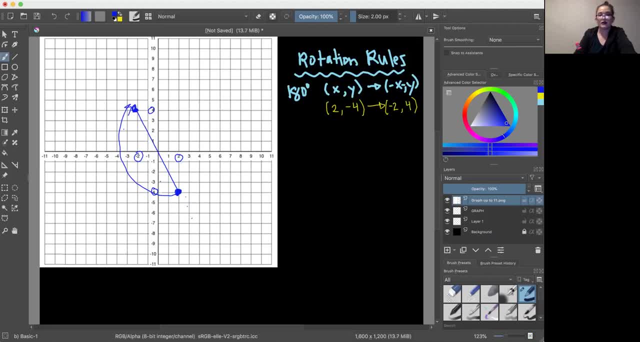 doesn't matter if you went like I showed you right now- counterclockwise, or if you're going to go or sorry, this way is counterclockwise. the way I showed you the first time was clockwise. but it doesn't matter which way you go, because 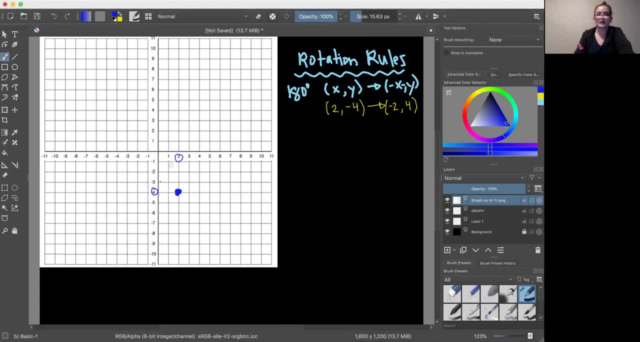 you're gonna get there either way, but that is kind of just an example of what we're talking about here, and I also want to write down the three things that you need to have in order to perform a rotation. so I'm just going to put need. 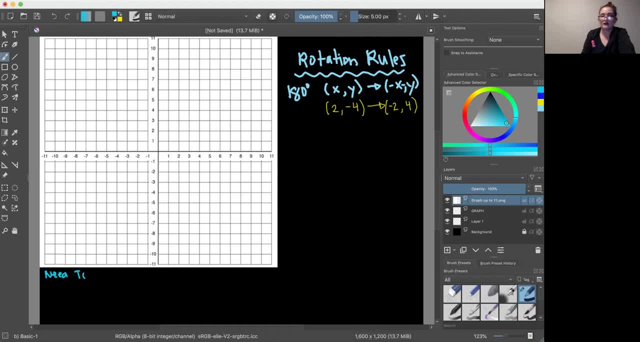 and to have. and again, if you're taking notes, write this down, okay? so in order to perform a rotation, you need to know the degree in which you are performing the rotation. so a 90 degree, 180 degree, what degree are you moving? and then you also: 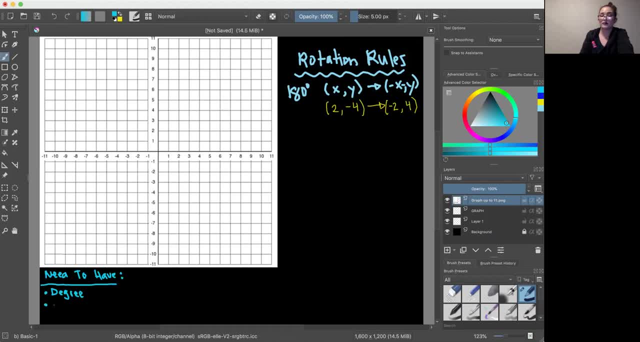 need to know the, the direction, okay. so are you going counterclockwise or are you going clockwise? and the last thing that you need to know is about. sometimes people say around what point? so a really common one is around. or about the origin and the, or it could be a 90 degree counterclockwise rotation about point A. So either you can. 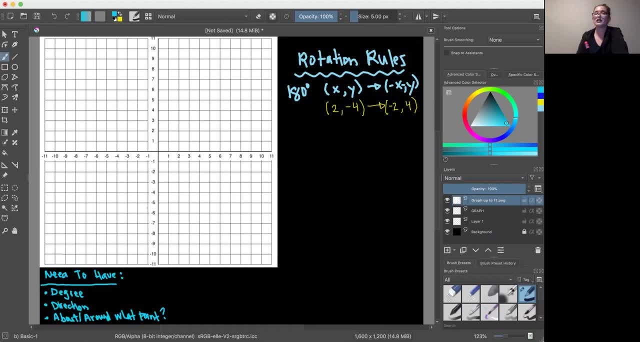 rotate around a point or you can rotate around the origin. Those are the two main ones that we usually see in seventh, sixth and seventh grade. But that, or sorry, sixth and seventh, I mean seventh and eighth grade. So that's that. Sorry, if you can hear my cat One. so right here we had 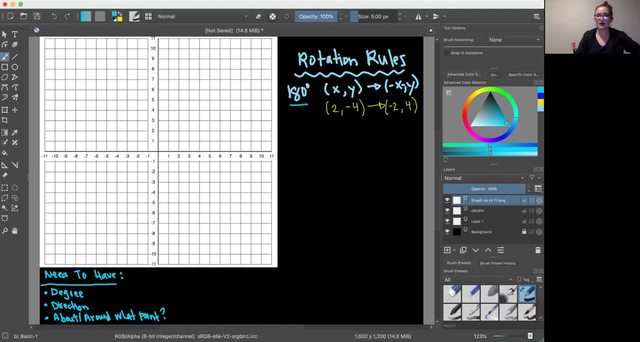 the degree. we had the direction, it doesn't matter- with the 180 degrees. and then we had about the origin. It was the example that I showed you. So the next rotation rule: I'm going to do a 90 degree rotation. The direction is going to be clockwise. 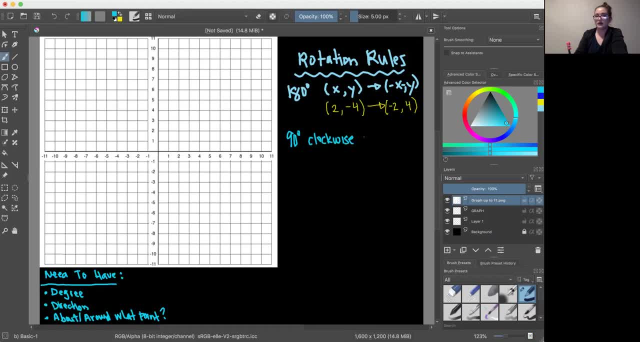 And then about the origin is my example, but this rule can work for any around or about any point. It's not just the origin, so I'm not going to write that here, But basically what it says is: you start with any point- X and Y- okay- and then you flip the X and the Y point. 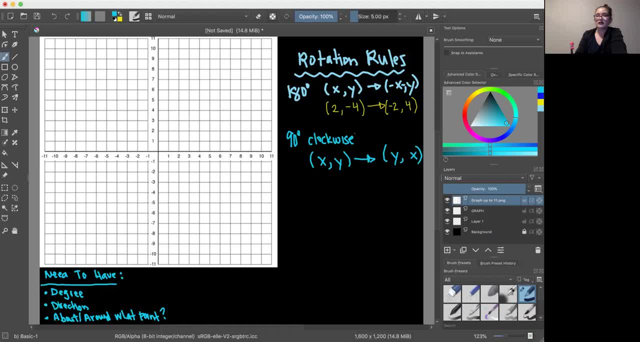 Okay, and clockwise means that you're going to the right right, So I'm going to put an R right here for the right. So the way I remember this rule is that my right number has to be opposite, So I'm going to take the opposite of X or my X number. This is in the 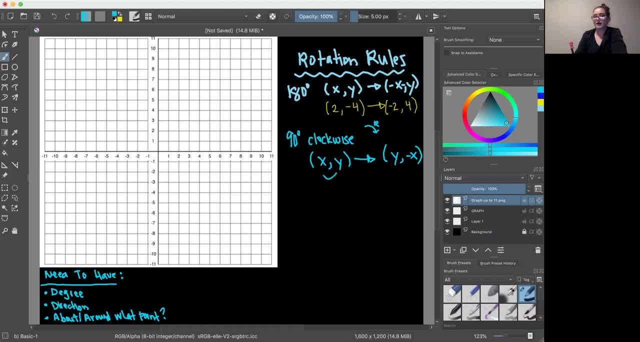 Y location. but you know what I mean. So we switch, we flop the X and the Y, we switch those locations. So my Y number would go first And I think it would make more sense if I showed you an example. So let's take a look. If I had the numbers, let's say four comma three as my point. 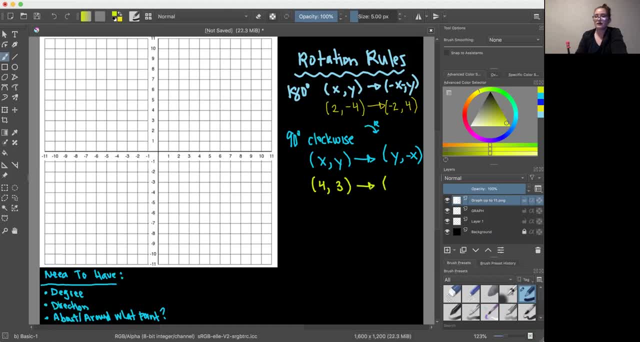 then my four and my three would switch places. So my Y would go first and then my X, but I'm going to make the X opposite, So instead of a four it would be a negative four. Okay, these are my new X and Y coordinates. Okay, so let me show you, with these points, the example. 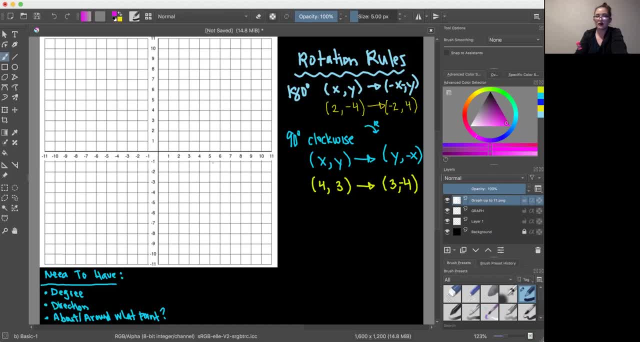 So again, let me change my color here so you can see it better on white. But my original point was four comma three, So it was this point right here. And now my 90 degree counter clock, or sorry, my 90 degree clockwise, clockwise around, or about. 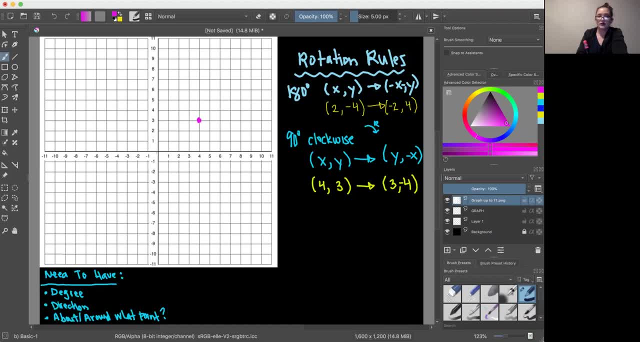 the origin. my new point is going to be three comma negative four. So right here. So if this was our original point A, this would be the A prime. Okay, and I know it's 90 degrees about the origin, because if I draw a line from that point, the original point to the origin. 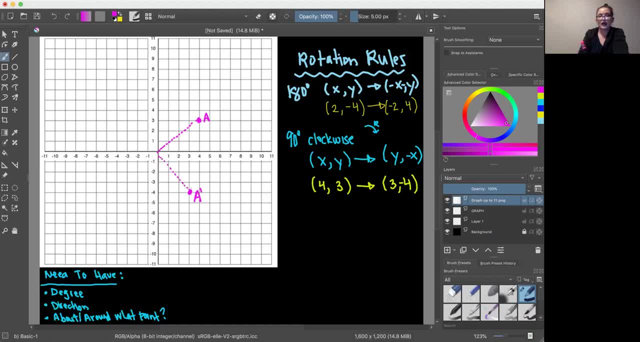 and then the origin, to my point prime. I have a 90 degree angle here, Okay, and I went clockwise, right? If you went counterclockwise it would be a 270 degree rotation, counterclockwise, But that's we're not looking into that right now. So that would be the example for the 90 degree. 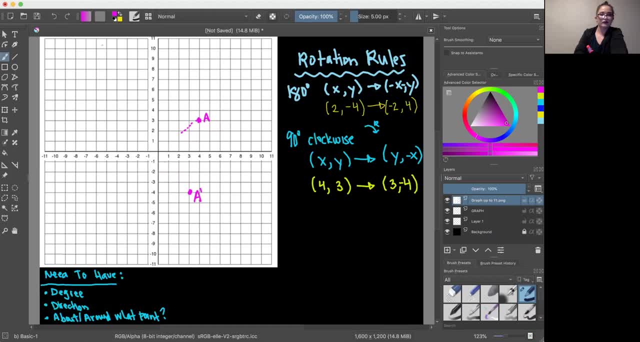 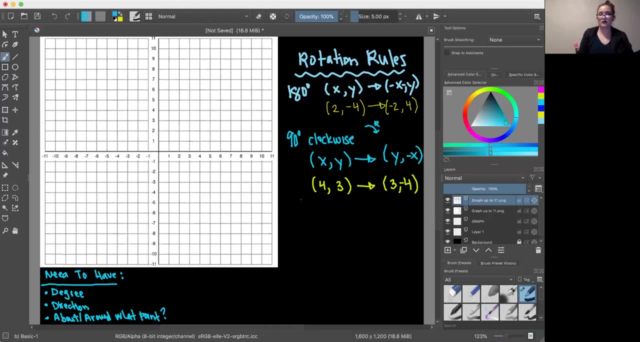 clockwise about or around. So we're going to call this point the origin. Okay, Um, let me see. Alright, so now that we've got that erased, we are going to now take a look at our last rotation rule, which is a 90 degree counter clockwise. 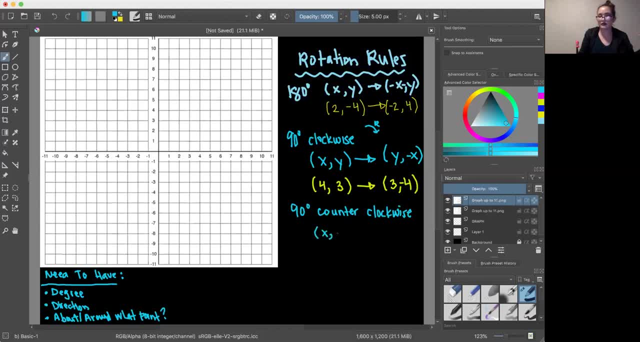 Okay. so again, if I start out with any point, my X and Y point, it is going to flip, just like it did for the clockwise. so my Y- let me just move that over a little bit- my Y is going to go first and then. 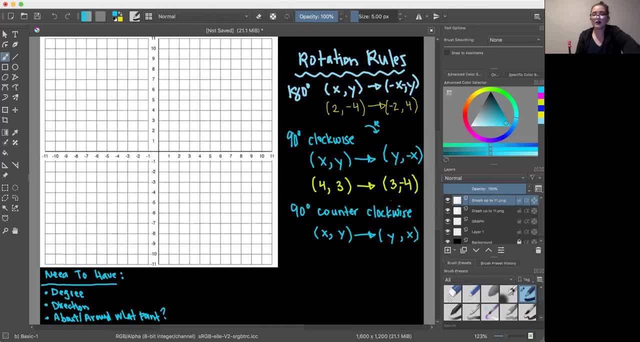 my X. okay, but this time counterclockwise is going to the left this way right, and I'll put a little L right there to represent counterclockwise is going to the left, and so for this new point, it is my left number that is going to be. 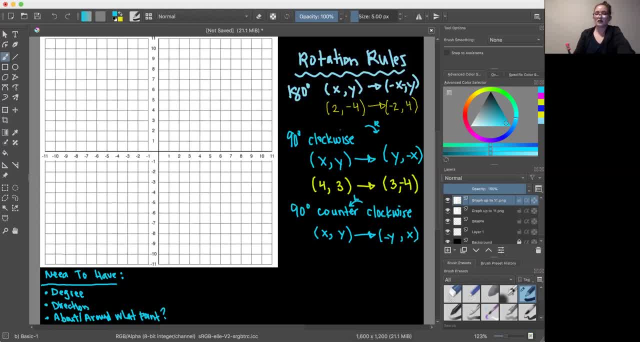 opposite. so remember when we talked about the clockwise, this is your original point here and this is your image point or your point prime, and it was the right number. so in both clockwise and counterclockwise you're flipping the X and the Y for the new point. 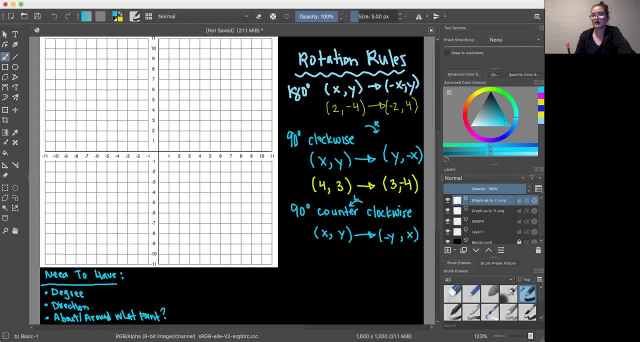 your Y goes first then your X. here, counterclockwise, your Y goes first then your X, and the only difference is when you go clockwise to the right, the right number gets the opposite. when you go clockwise or counterclockwise, which is, to the left, the left number gets its opposite. it's turned into the opposite. 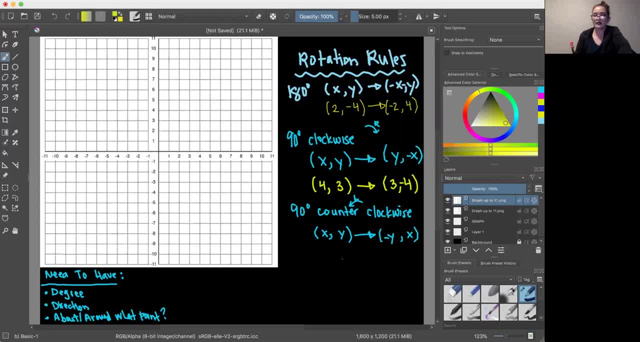 so let's take a look at this one as an example. this time I'm going to say that if I had negative numbers, so like say, if I had a negative 1 comma, negative 3 as my original point. moving to this new point, 90 degree counterclockwise. 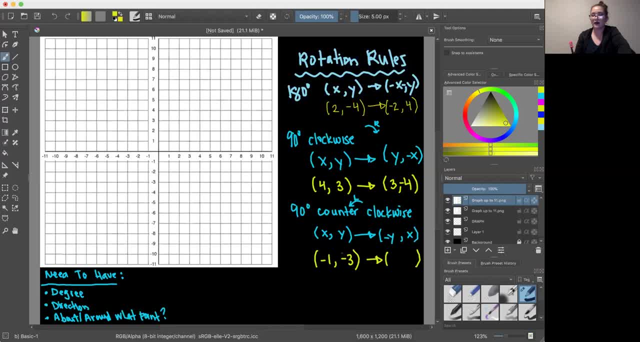 rotation. I'm going to flip, so I'm going to put my Y first, which is negative 3, and then my X, which is negative 1, but I'm going to take the opposite of my Y. so instead of a negative 3, it's going to be a. 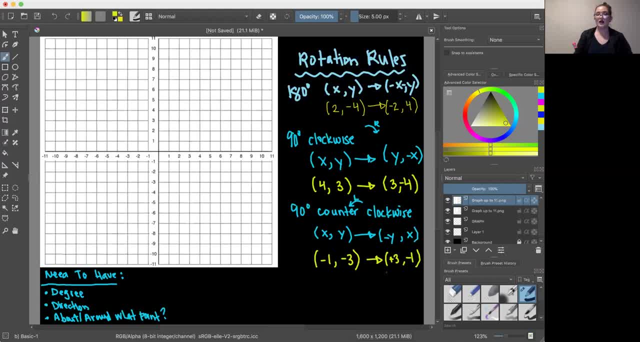 positive 3. okay, and so to plot that as an example I am going to, my original point was negative 1, negative 3, so let's just call this a and again, this is around the origin that we're doing the example for. so the new point, or the point prime, a prime, would be positive 3, negative 1, so this: